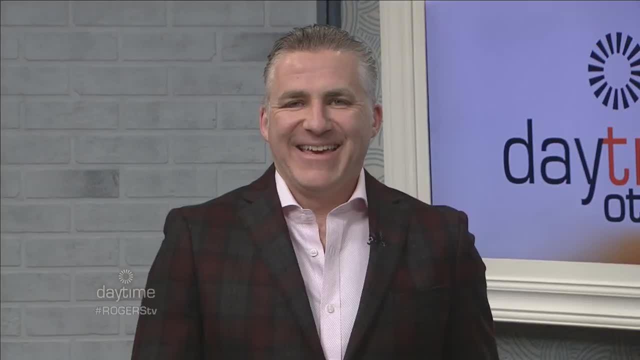 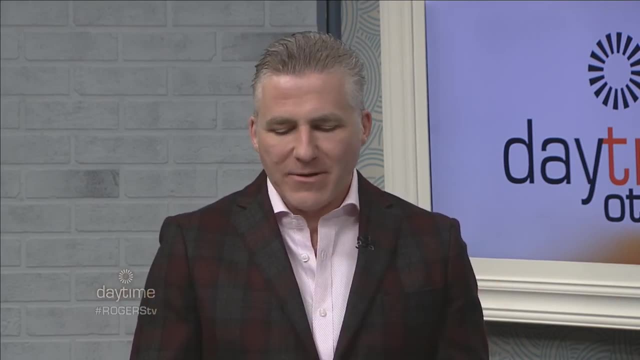 And he indeed is the organizational coach. His name is Steve Gingras. He always drops by to help out with many aspects of our life. This time around, we're talking about time management- Very important, Hello Steve. how are you? Thank you, Dylan, for having me, and this time it's for. 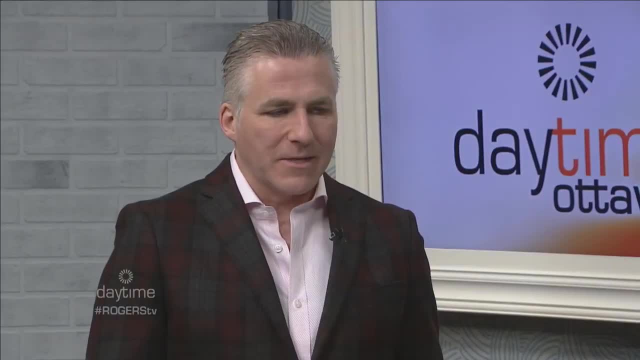 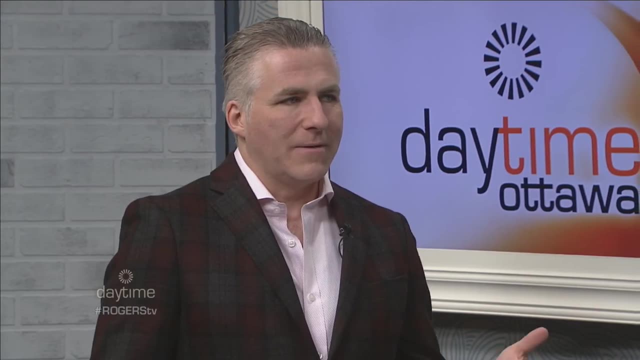 children For children this time around, which is good, because kids sometimes lose track of time, and we'll talk about why they do coming up. Where is your love for time management organization? Where does this all come from? Does it come from your childhood? Yes, like my parents were very. 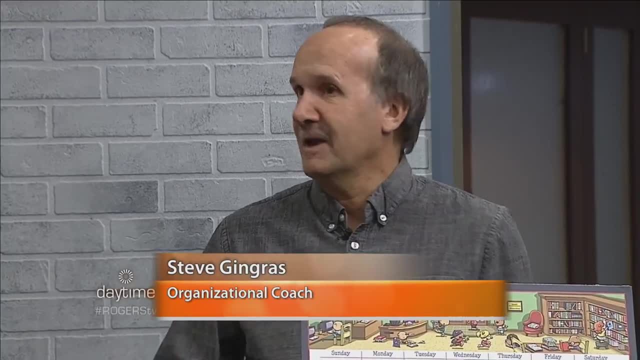 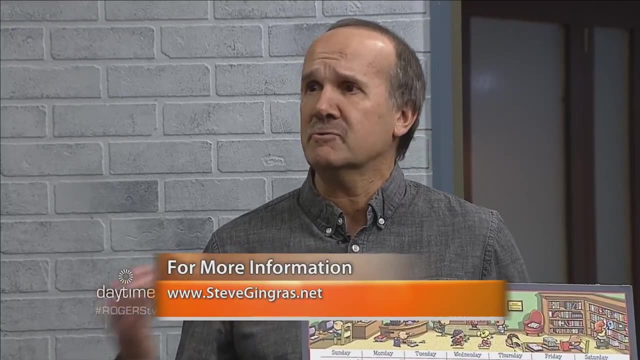 strict on, let's say, if you had to make it someplace- that not to be late for school, not to make sure that for sporting events that you're not late and the coach gets mad at you, and everything like that too. So I just had an interest in that too, and then, when I was in my very early 20s, I started. 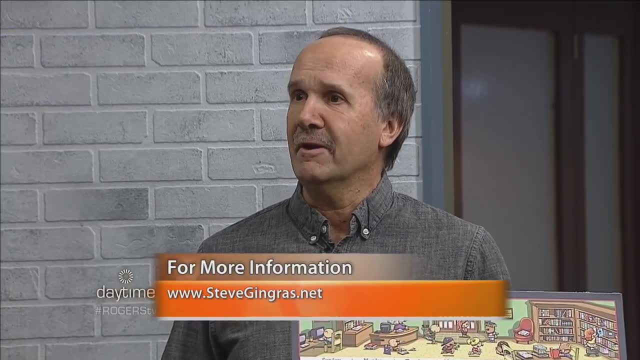 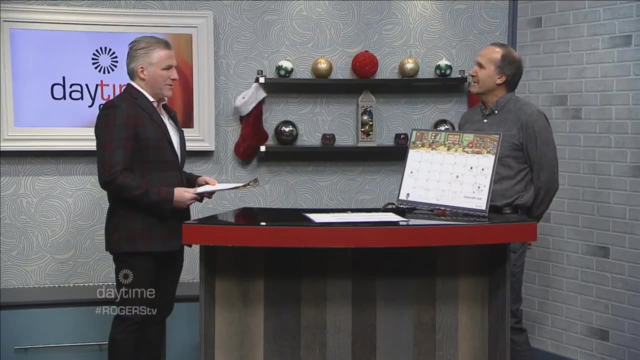 doing competitive coaching then and I just found through that then the more discipline I offered to the kids there, the better they enjoyed it there. They excelled probably too Some. Some teams did, some didn't. Talent had a lot to do with it too. Okay, we're talking about 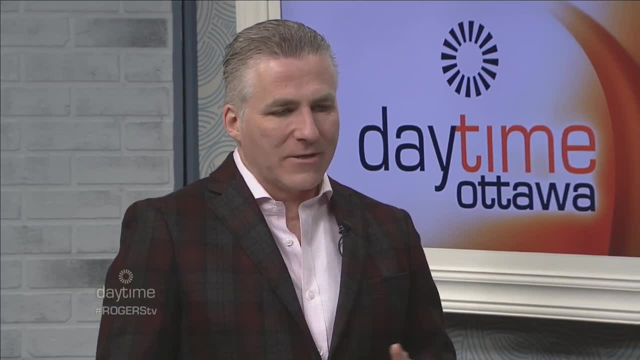 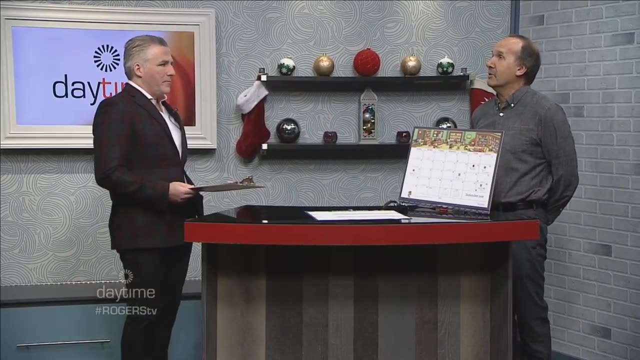 age by age teaching here as well. so you want to begin with three to four year olds? Sure, so I guess your son is what? two years old. Two years old, so he probably doesn't grasp much of this just yet, right. So he's kind of like the idea of, okay, can I do it now? Yeah, right now, or else Like does. 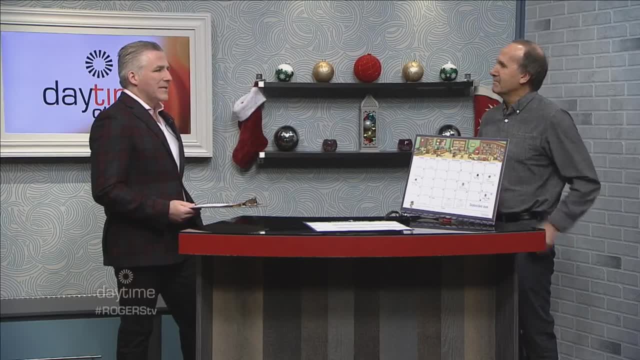 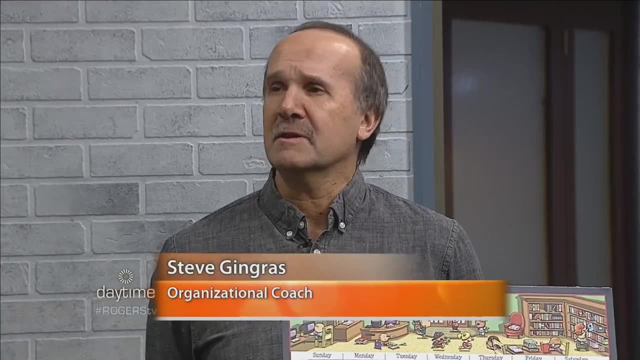 he know Christmas is coming up. I don't think so, quite honestly. I think like he's just excited about the moment. Right, Yeah, instant gratification, I think. Okay, and that's that's the thing. with the younger ones It'd be like kind of like that's the first thing we should be teaching them is like the seasons. 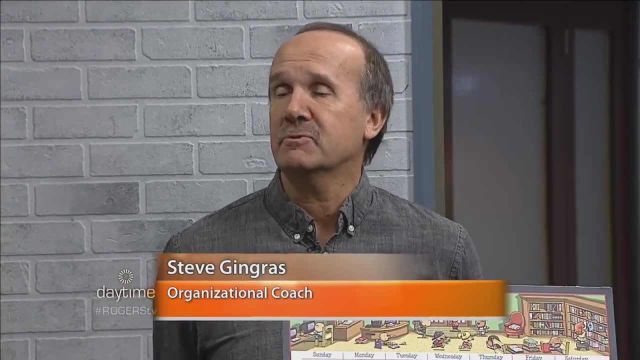 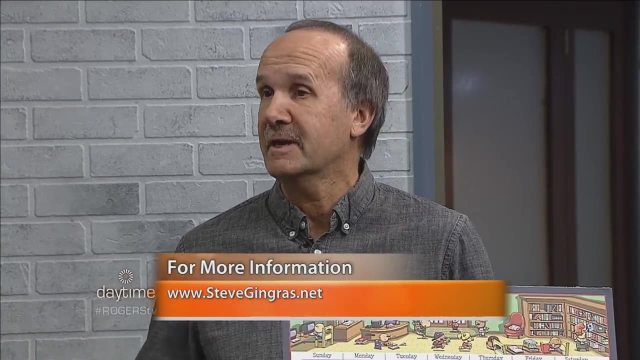 like now you're seeing winter, then in the spring that's like two. so it's a good thing for them too, and also the fact that introducing that events coming up that are a couple days later than not necessarily it's three weeks from now, because they would have no idea in terms of time what that 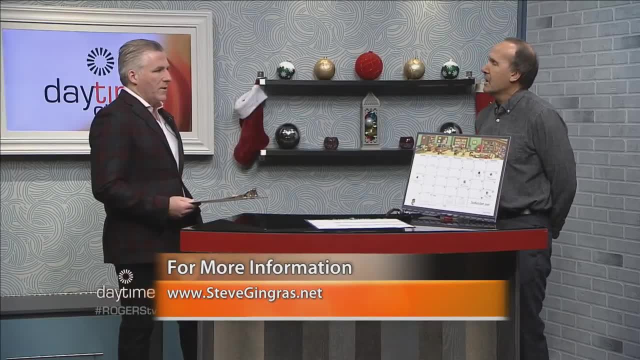 would be. Okay, so that's what the plan then. for what age would that be? for that? That would probably be, maybe just before you go to school. Okay, so when you get a little older, what's the best way? So the next one would probably 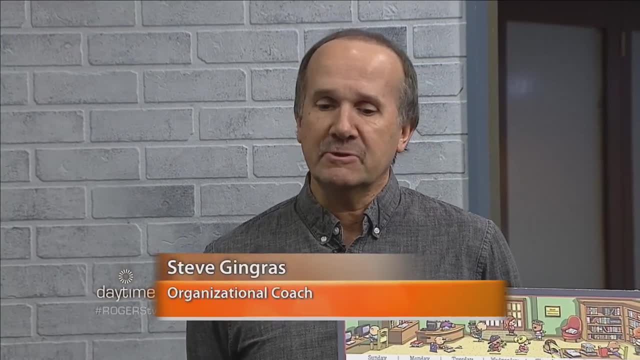 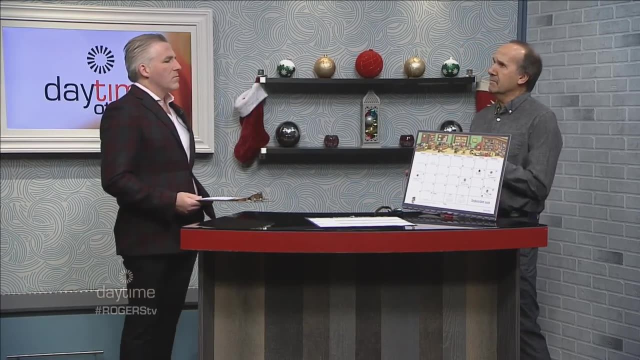 be like, let's say, your kindergarten and grade one age there, and then you're interest introducing them the concept of the clock and the time and everything like that too. so you're looking at that to say like um, um, you're gonna schedule something like this too, and it's gonna be like uh, let's say 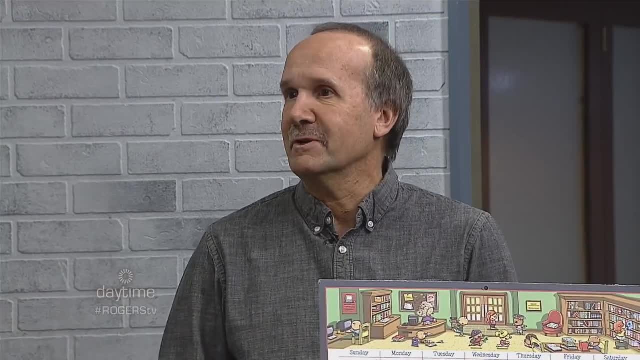 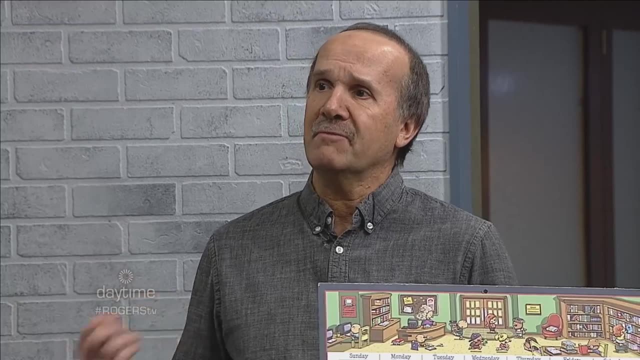 for example, you're doing your, you'll do your whatever homework they're doing in grade one then, for, let's say, at seven o'clock or something like that, so they're able to do that. so they're curious with time there too, and also the fact that saying if they don't make a certain time, then they're 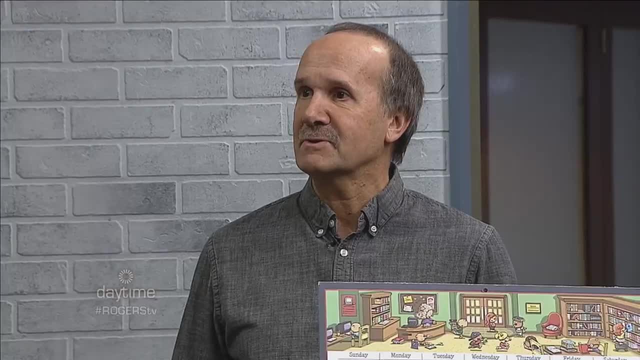 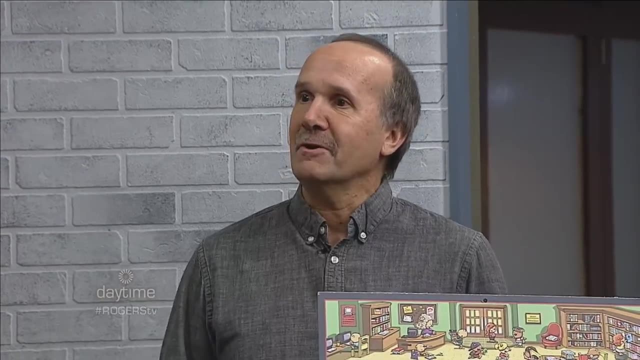 going to be able to do that. so they're going to be able to do that. so they're going to be able to do that. for example, if you have an assignment at school, even if it's grade one, then it needs to be done. if you, if you, if you're on a soccer team when you're five years old and you show up late, all 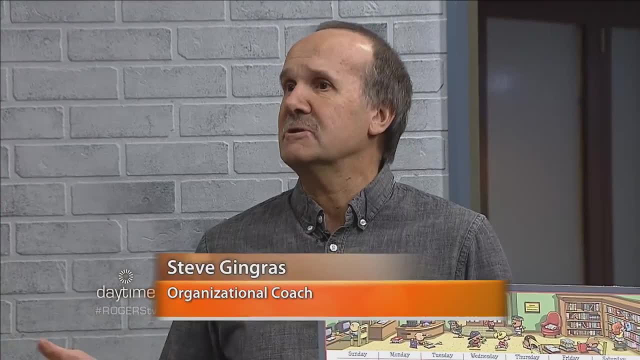 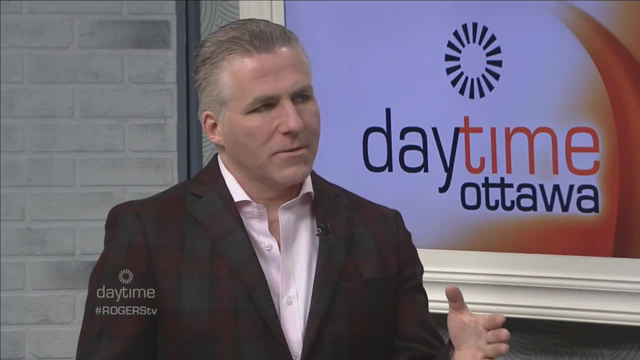 the time, the coach will not be particularly very happy. so it's just introducing the fact that there is consequences with Okay, and then obviously they will take these skills learned and developed and take them into their later years. That's, that's right then. so it's never too early, okay. so example: 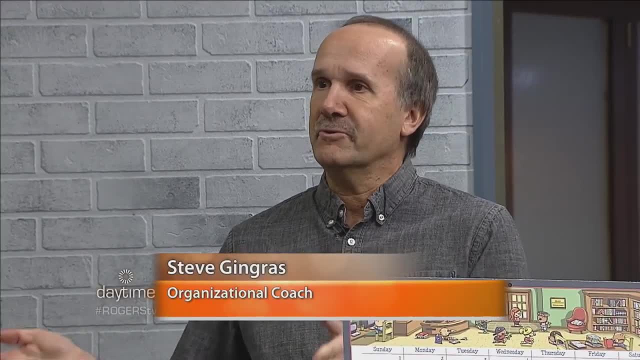 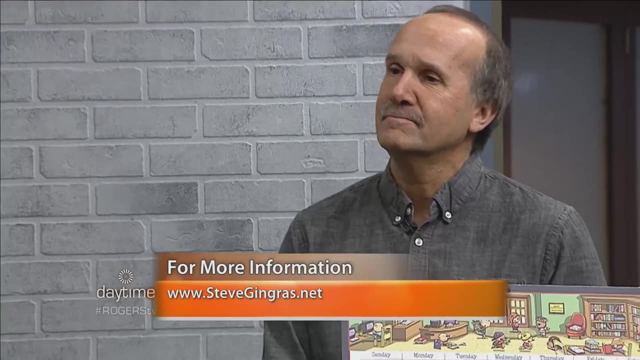 like even for your son being that young, then even introducing the fact that, uh, everything is not just here now, then it's sometimes a couple days later. then okay, good tip for me for sure, over scheduling your child is, is that a bad thing to do? yes, because i've had 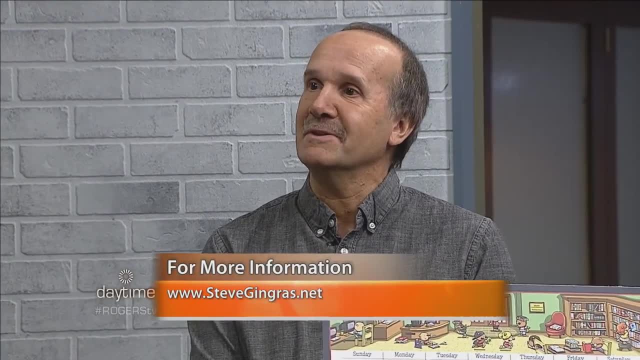 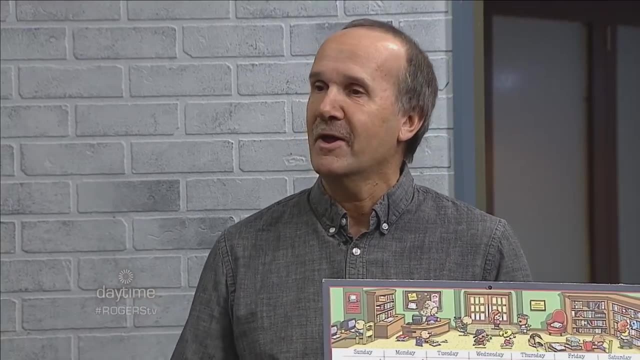 especially some friends there that actually have their kids scheduled seven days, seven days a week. then let's say, you go to brownies, then it's language lessons and it's music lessons and it's sports and it's like everything like that too. they've got them everything like that so. 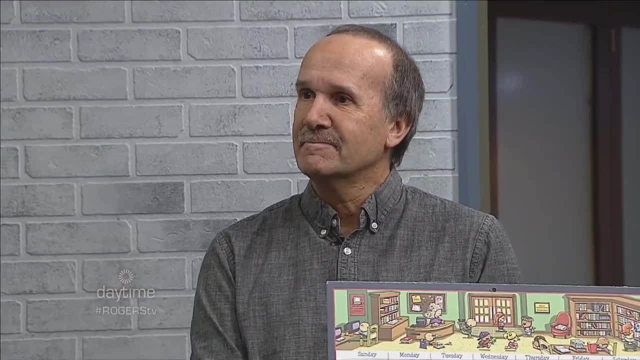 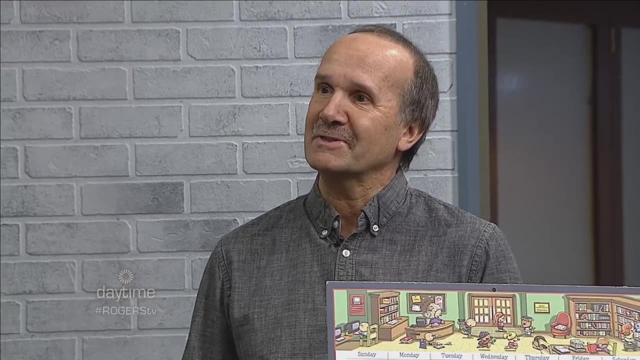 they actually have no time to actually be a kid. yeah, exactly, they need some time to just relax, yeah, and actually actually enjoy themselves. and a lot of times it's not, it's we're being forced into it. it's not like sort of like saying: guess what we find you up for. 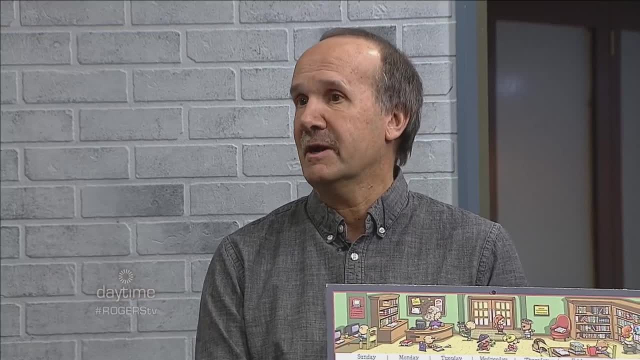 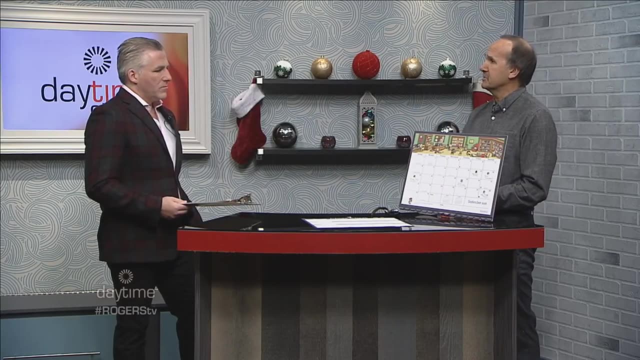 now, dear, yeah, we've sent you into this and we know you're into this. now what about some uh, teaching aids? uh, for teaching needs? i have one right here. then, for example, there are two um, uh, kids love things that are visual, especially the younger ones. then this one actually attaches to a um, 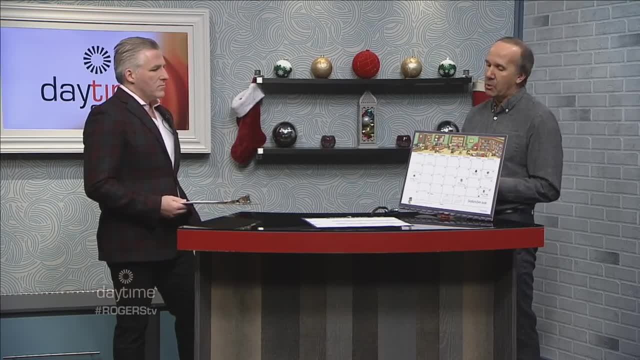 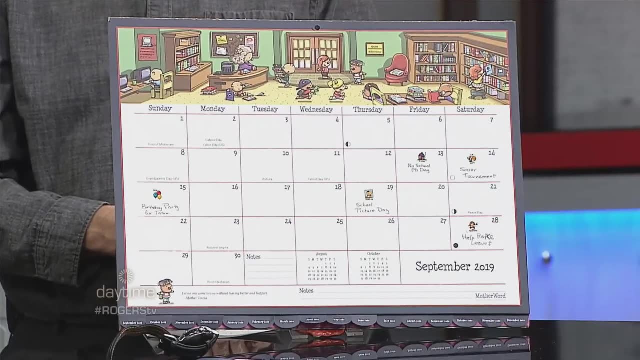 refrigerator then. so you can see like i'm using stickers and i have small ones there, but you can put some really bigger ones in. for example, let's say, in the 13th we have a pd day, on the 14th you have a birthday party, on the 15th, 19th has a picture day at school, and the 20th you're helping. 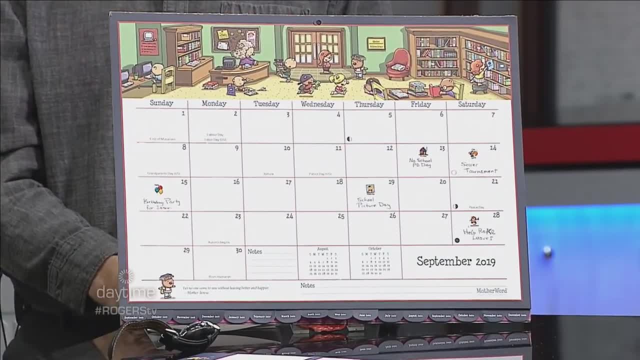 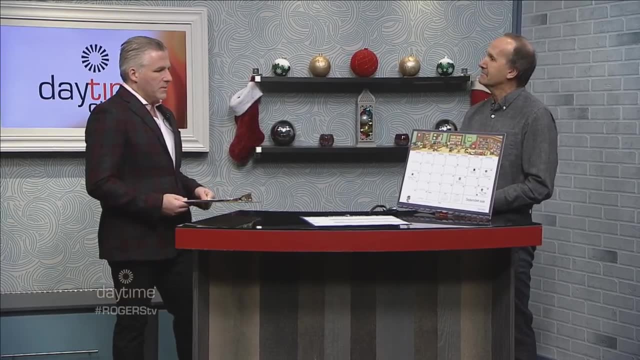 rake the leaves there. so it gives the kids like, let's say, a visual thing. they can put that in their room or on the fridge or whatever like that. so they immediately know, bam, they're ready to go that day. this is what's going to be happening that day. it's nice when it's colorful as well. 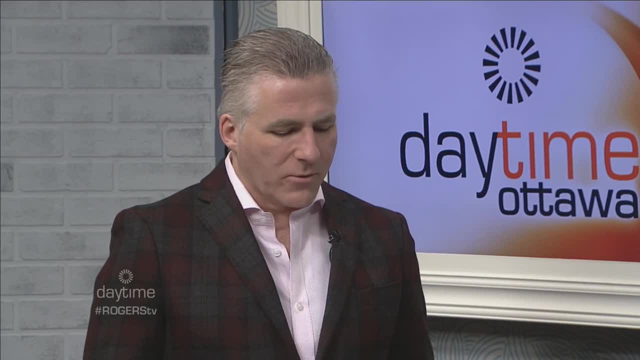 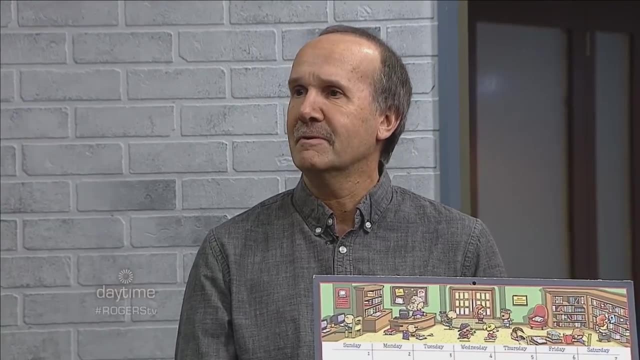 as you mentioned, there's stickers that oh yeah, yeah, very visual, so it's just like, and they can help participate in that too. then too, so it's also cute. it's key to let them have a say in what they're. why is it so important to let your kids help with the time management? because it's actually 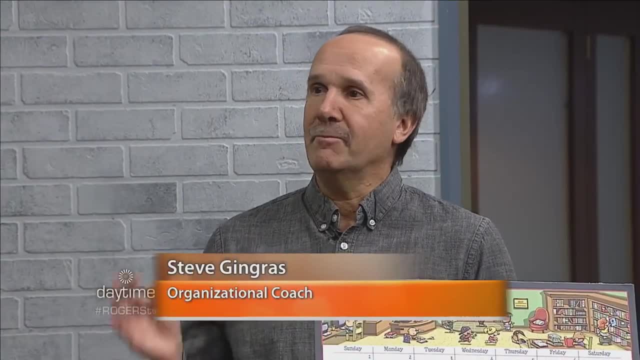 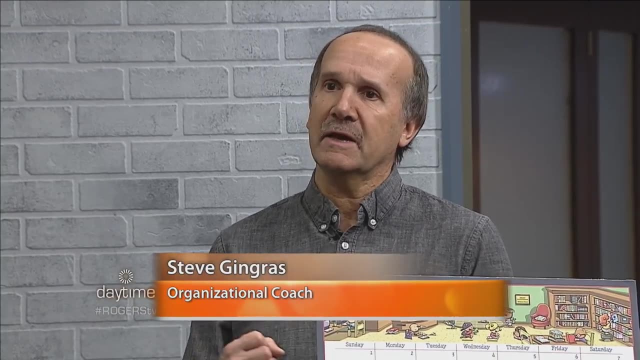 they play part of the role of family. there too, it's not just saying mom, dad or parent or whatever like that, or guardian just tells them exactly what to do. then it's like they have a say with that too say, and they also can say like i do, like late raking leaves, or let's say, when it's uh, recycle. 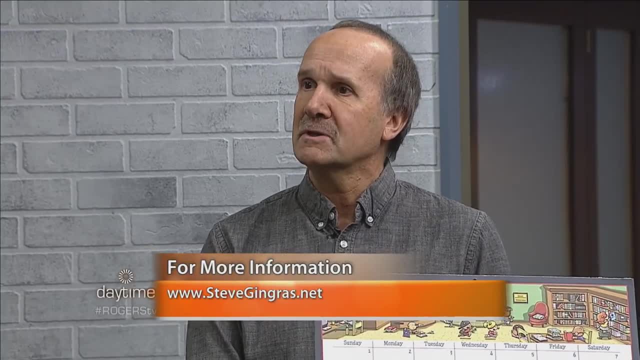 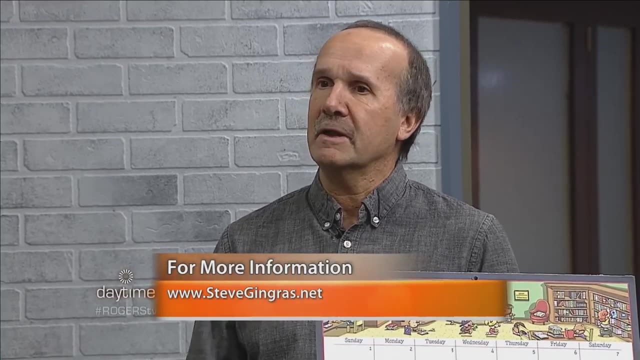 day. on thursday night, that would be your task to do there. okay, so, and then they can also work into the fact that they know that, um, when i do recycling on thursday evening, then it'll only take me. it takes me 10 minutes, so it gives a little practice with time. have you actually ever heard a kid say: 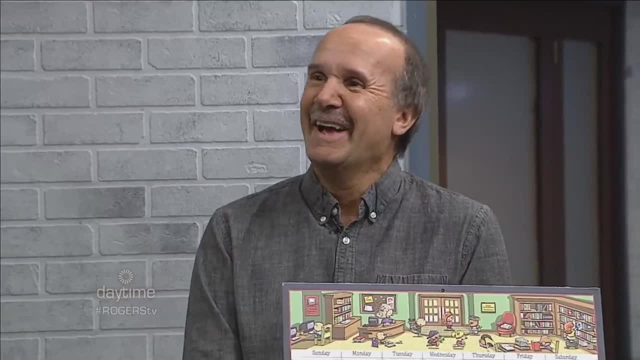 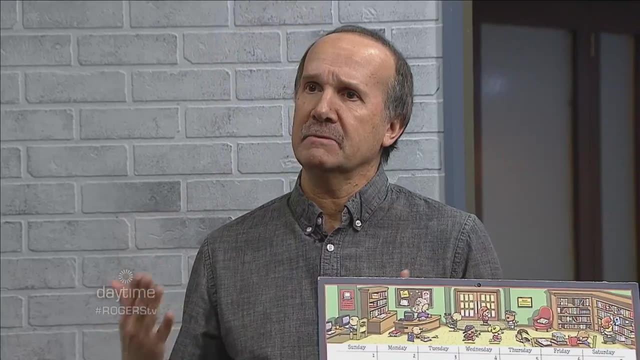 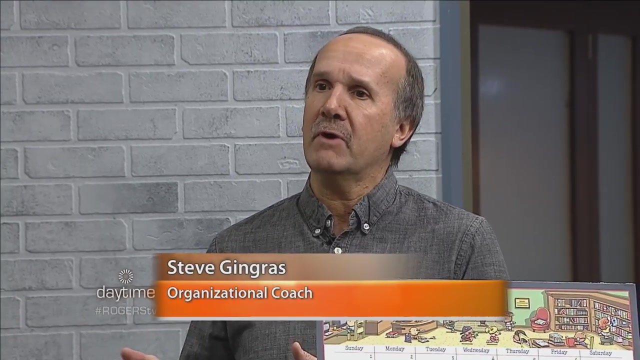 raking leaves. what about homework helpers? homework helpers is saying like, let's say, for most people would be like hopefully you can have it right after dinner you do your homework, or just before there, and also to having the support of your parents there and also the fact to having a nice area to do. 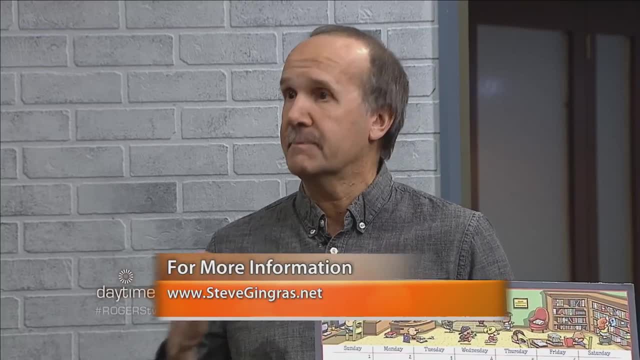 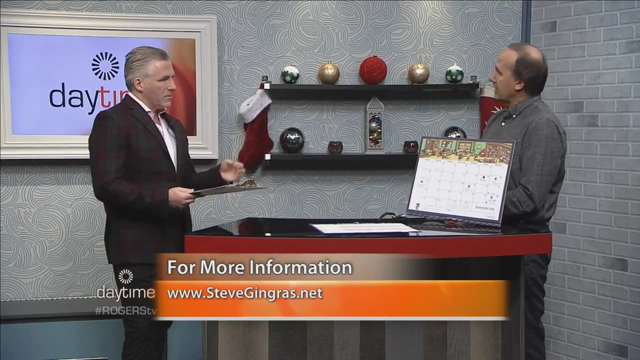 your homework to like an isolated area just for them then, and supporting and bearing a cheerleader for your kid and everything like that. okay, coming up in 2020, you're gonna have more workshops and they're gonna be focusing on children. yeah, I'm going to be born that because there seems to be more and more. 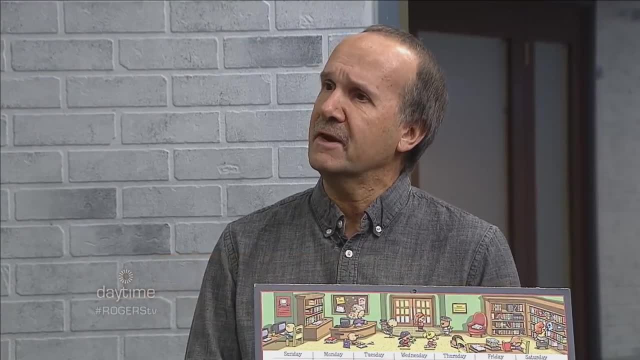 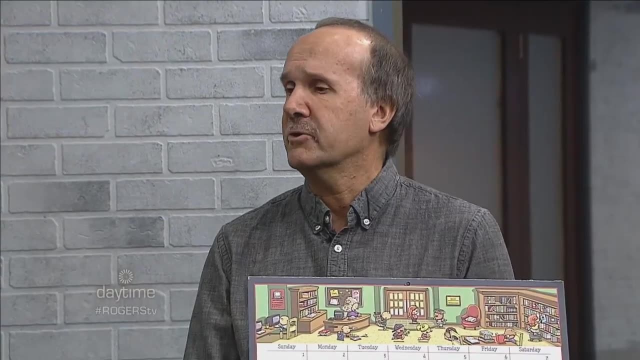 interest of that too, because, especially to there's so much to do for kids these days, so I think it'd be a good help if they started really early. I did have a class I did a couple years ago where a mom brought a 12 year old kid with her. 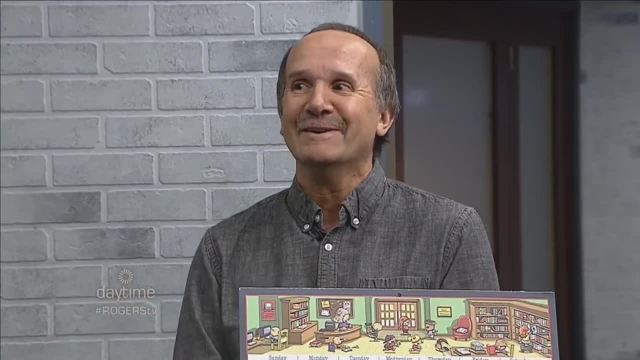 and to actually try it. for a 12 year old to do that it's a little bit too much. totally okay, Steve Shingrod dotnet, for great things in the new year. thank you very much. thank you, don't appreciate your time coming up. big soul project. what it's all about next time, Rogers television.